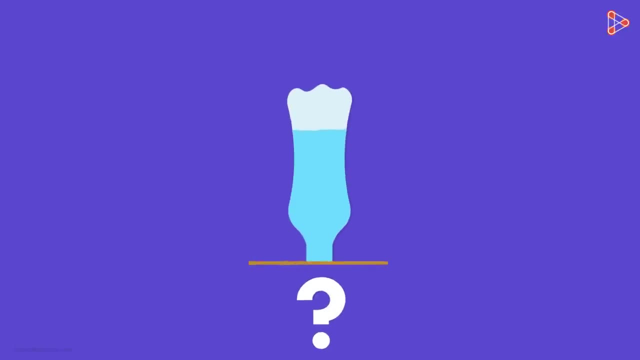 Now take off your hand from the cardboard. What did you see? The cardboard sticks to the surface. This is because the air's pressure is pushing the piece of cardboard in the upward direction. Does this mean that air is heavier than water? Well, the air is present everywhere, and hence 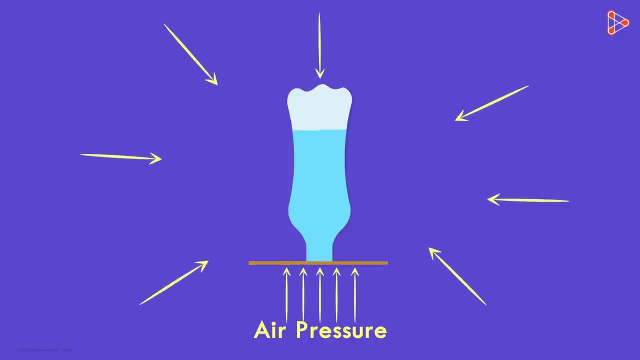 it's exerting pressure from all the directions. Clearly, the air pressure is more than the pressure of the water inside the bottle, And this allows the piece of cardboard to stay on the surface of the bottle. With this activity, we can understand that air exerts pressure. 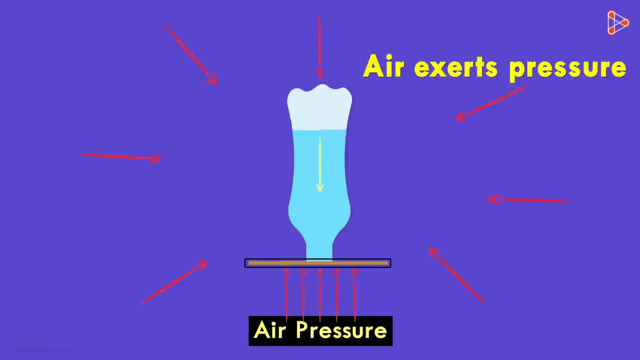 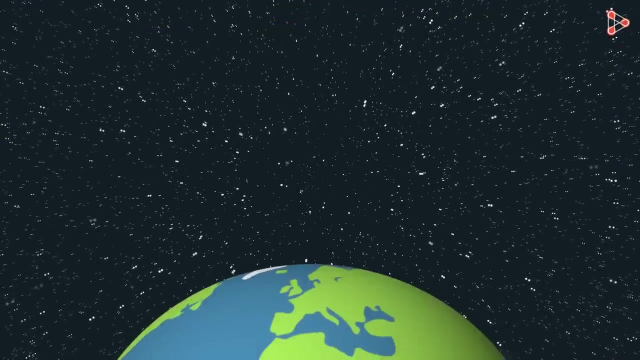 You may note that the air pressure acts in all directions. Do you know why? It's because air is fluid. The molecules of air are very loosely held and hence they can easily move in all the directions. We all know that the earth is surrounded by an envelope of air. Do you know what it's? 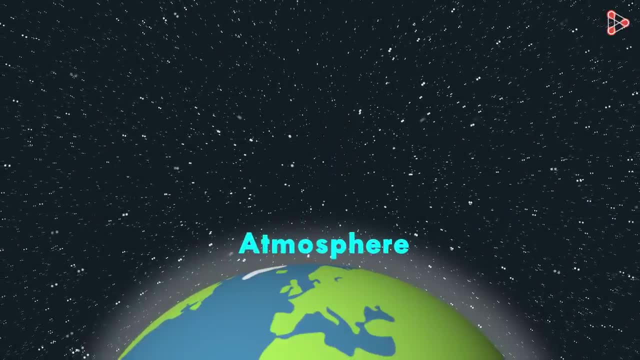 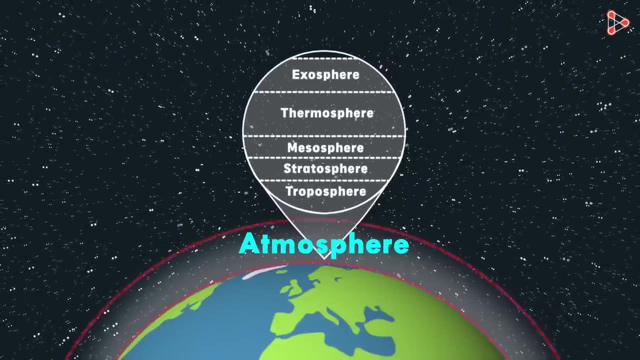 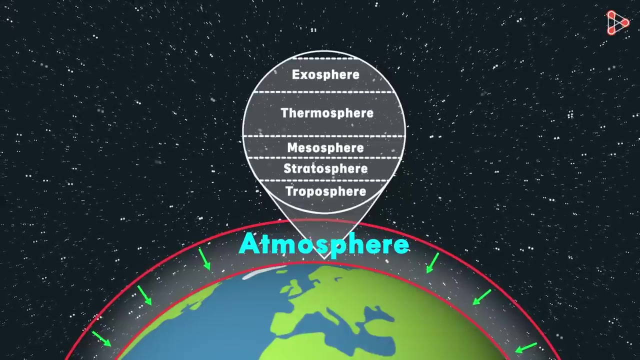 called. It's called atmosphere, And this atmosphere is divided into different layers, as shown in this image. What can we say about the air in the atmosphere? The air in the atmosphere exerts pressure on the earth. or we can say on the earth's objects What? 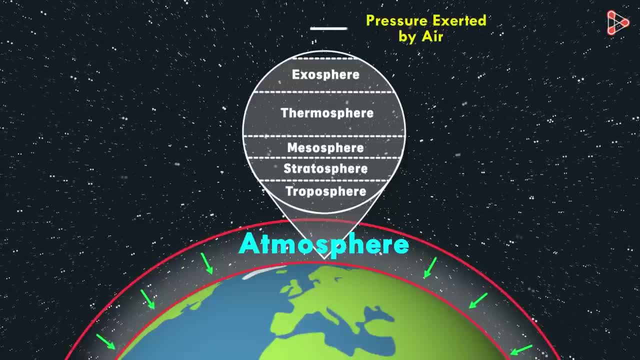 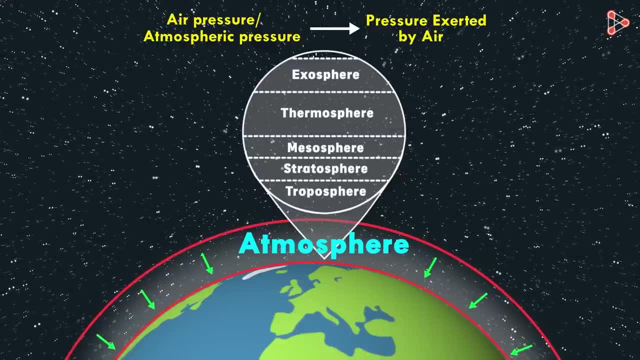 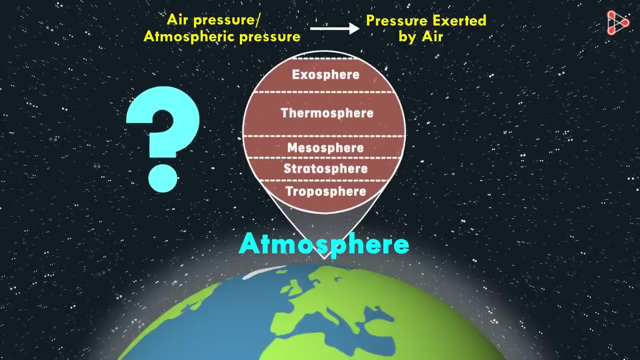 is this pressure called? The pressure exerted by air is called as air pressure or atmospheric pressure. Now the question is whether air pressure is uniform throughout these layers of atmosphere. Think about it. Where would the maximum quantity of air be? There is maximum air above troposphere. 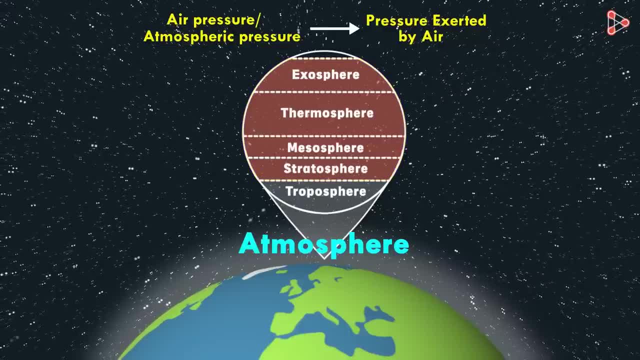 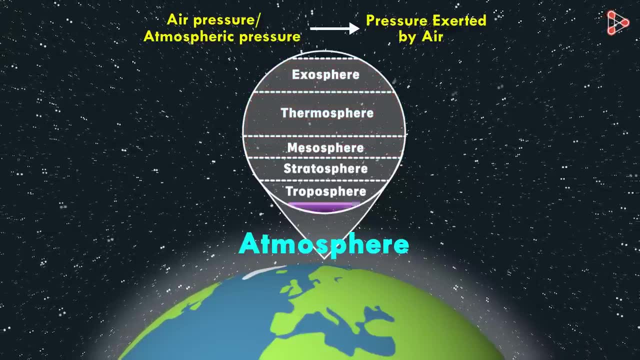 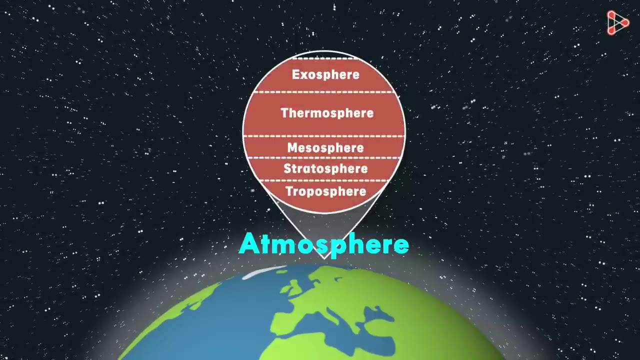 There's this much air above the troposphere troposphere, then this much air above the stratosphere and this much above the mesosphere, and so on. So as we move upwards, the quantum of air decreases. Now, logically, can you tell me which layer carries the maximum air pressure? 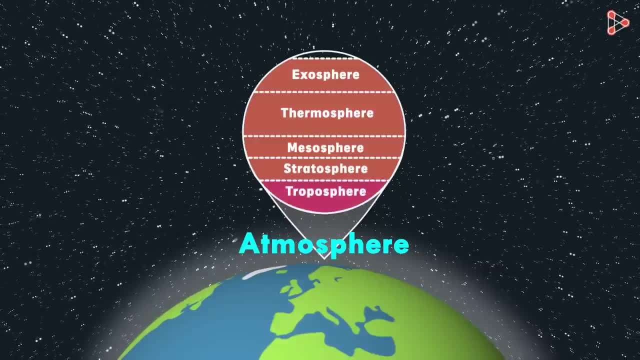 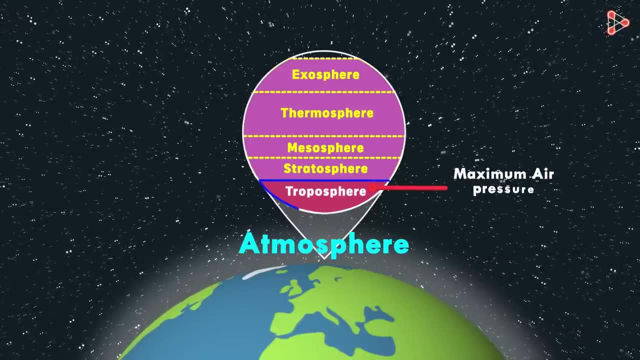 Yes, the bottom most layer carries the weight of the air present in all the layers above it And that's the reason why the air pressure is maximum at this layer. And what can you say about the air pressure at the layers above this point?